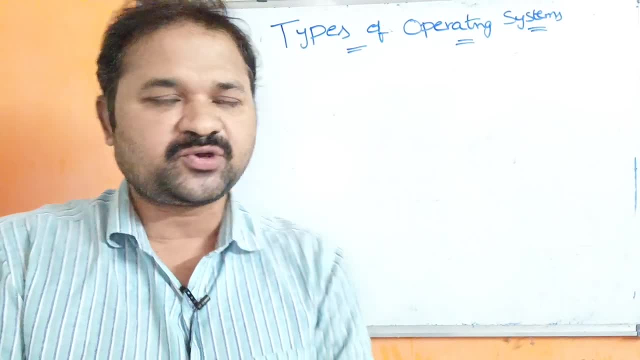 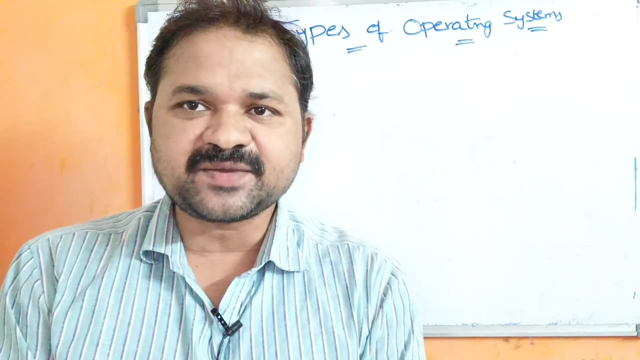 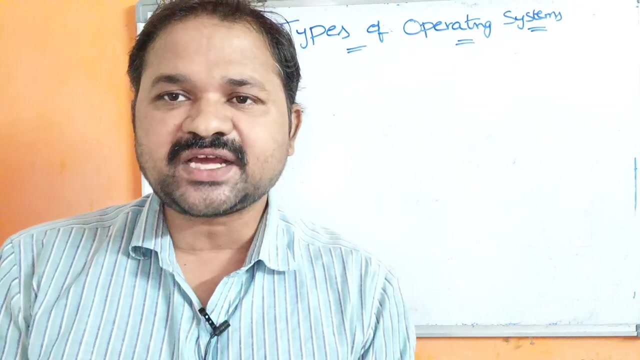 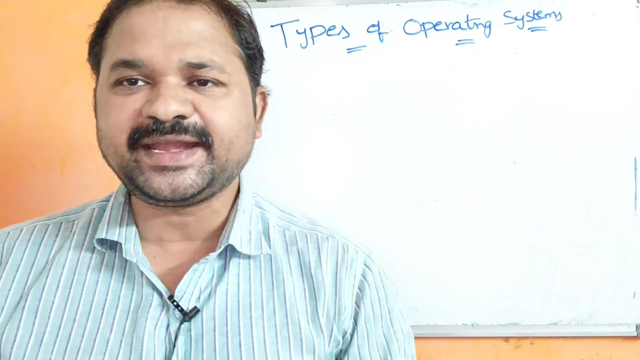 In this video we are going to discuss about types of operating systems. We know what is operating system. Operating system is an interface between user of the computer and computer hardware. Without installing operating system we cannot perform anything in the computer. Let us see about types of operating system. We have mainly seven types of operating. 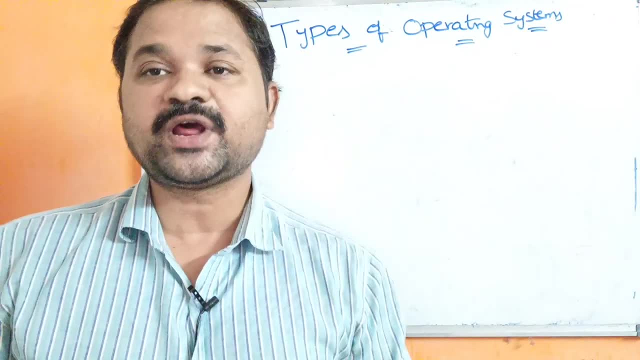 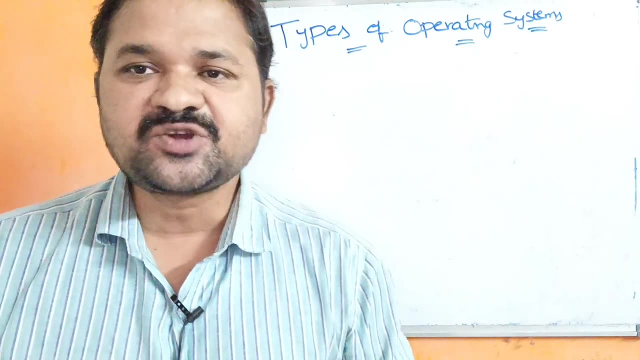 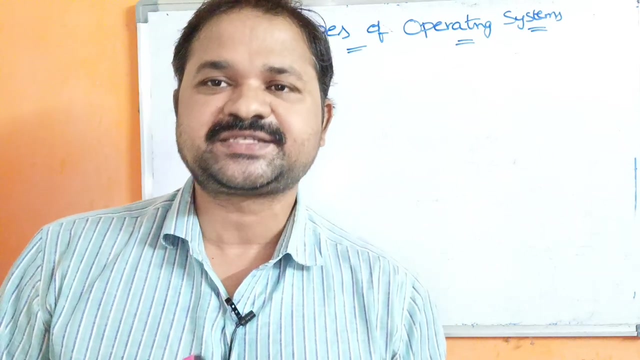 systems are there: Batch system, multi-programming system, multi-tasking or time-shared system. next one: multi-processor system, distributed system, real-time systems. These are the important operating systems. Let us see all these operating systems one by one. 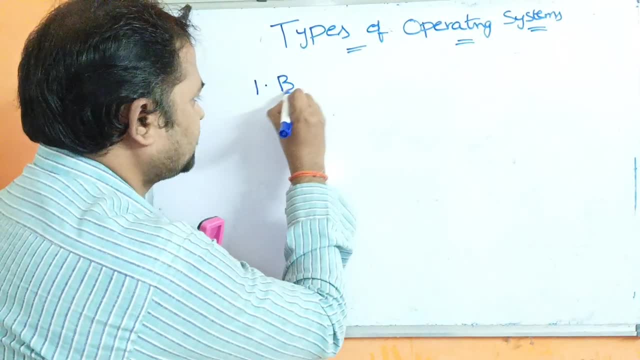 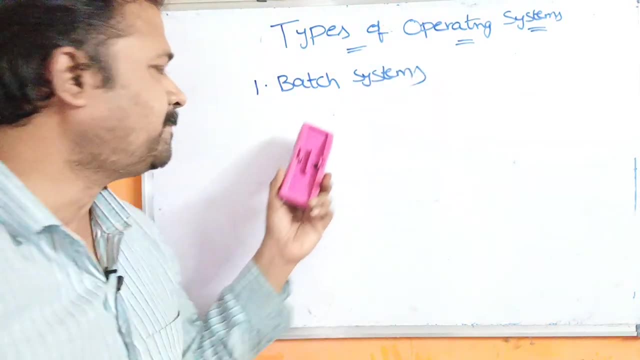 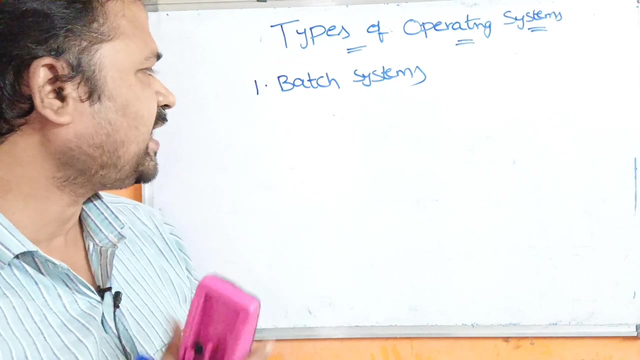 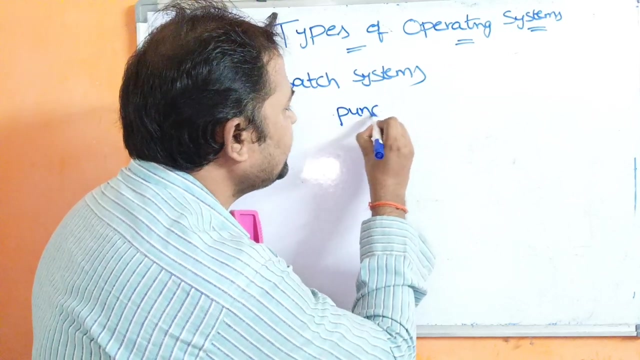 The first one is batch systems. The first one is batch systems. So what is a batch? Batch means a collection of jobs. In this type of operating system, what will happen is the user uses punch cards. So in the olden days we used batch systems, punch cards. 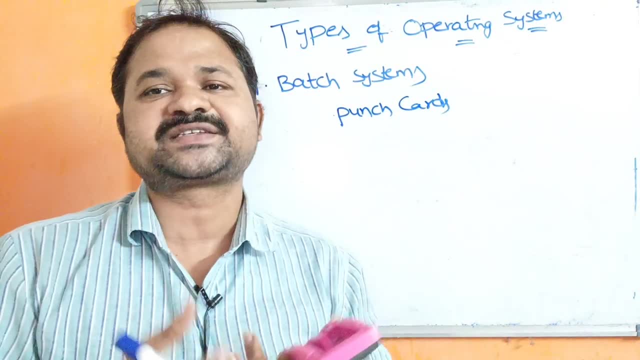 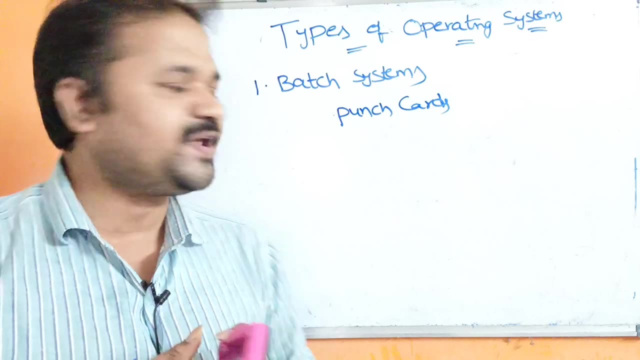 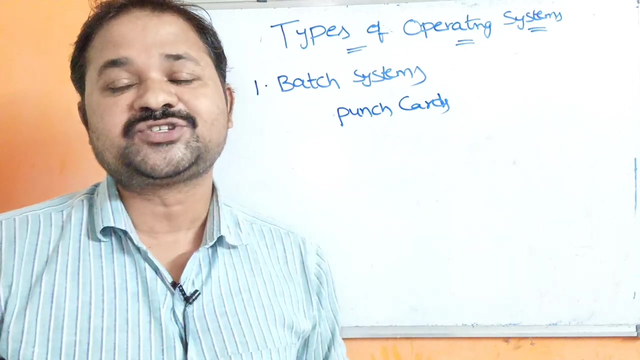 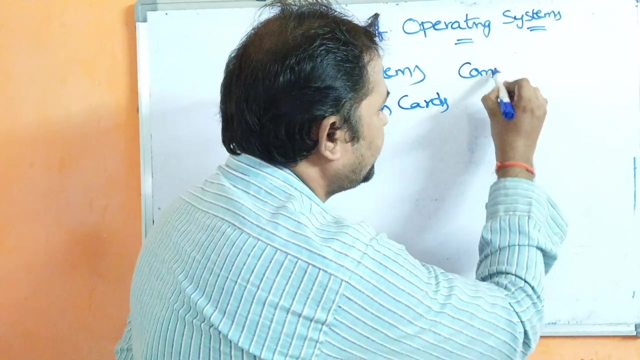 So here the user provides the program or job information in the form of the punch card, And after submitting the, after writing the corresponding program or job details in the punch card, all the jobs will be submitted to the computer operator. computer operator. here the problem with this approach is: 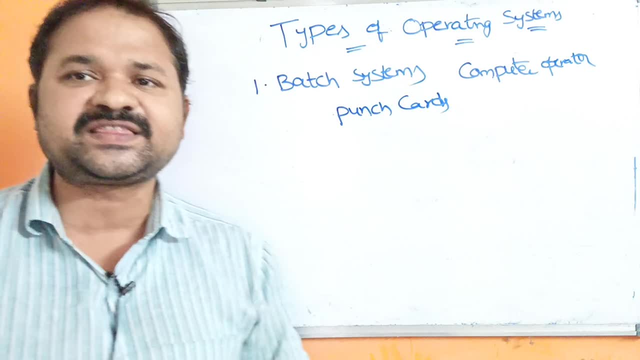 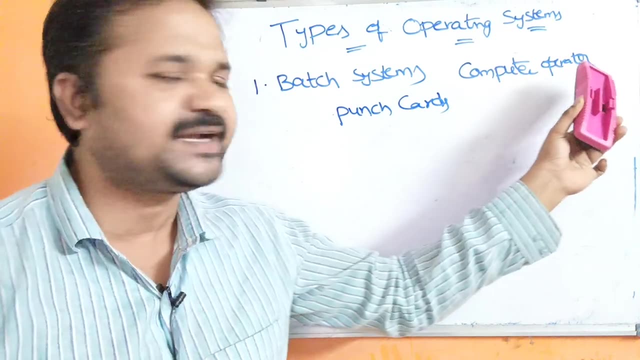 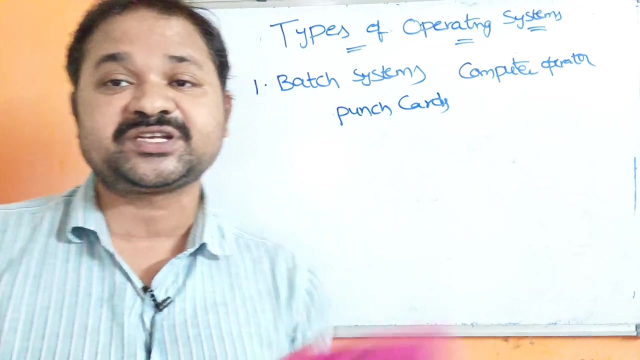 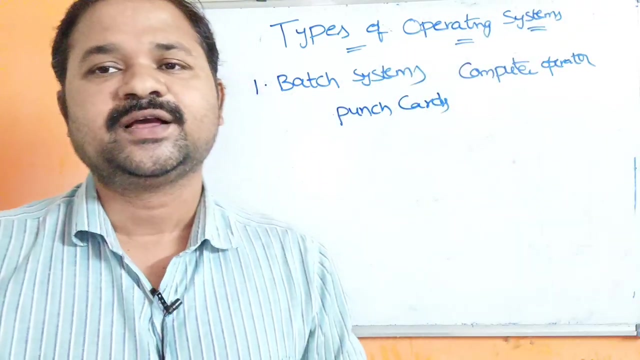 that the user cannot interact with computer directly. in between user and computer we have computer operator, is there, okay? so here first what the user will do. the user will provide the corresponding program information in punch cards. so once that information is written, once that program code is written, then all the jobs will be submitted to the computer operator. let us assume 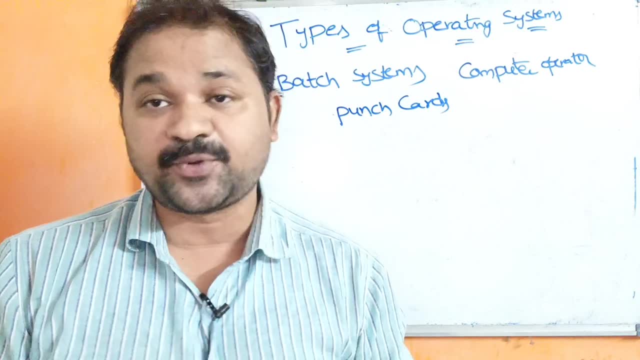 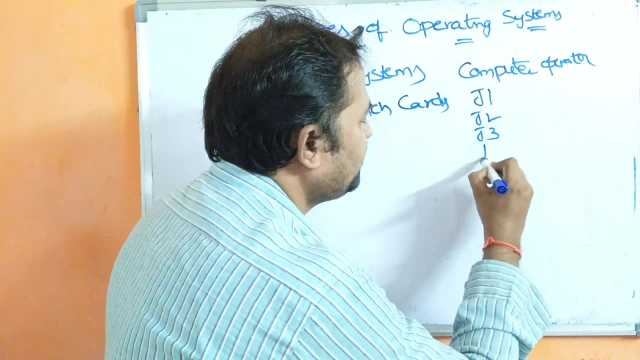 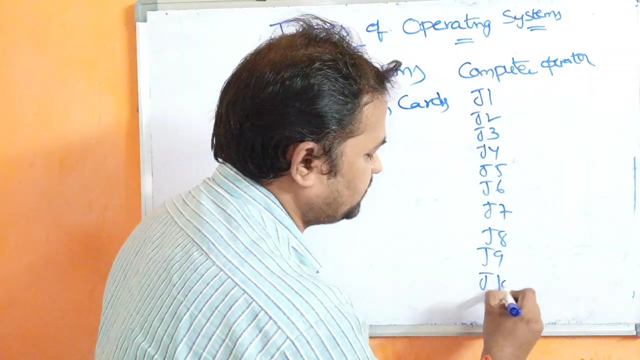 that user wants to execute 10 jobs or 10 programs. so, in the form of punch card, all that information will be supplied to the computer operator. computer operator: okay, computer operator- okay, let us assume that user wants to execute 9 job, 10 jobs, okay. so here all this information, all the program information will be available in the form of the 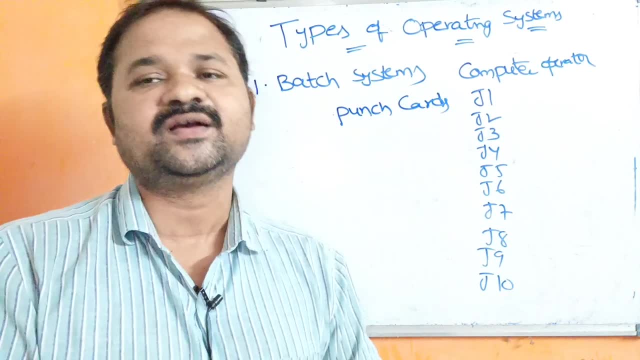 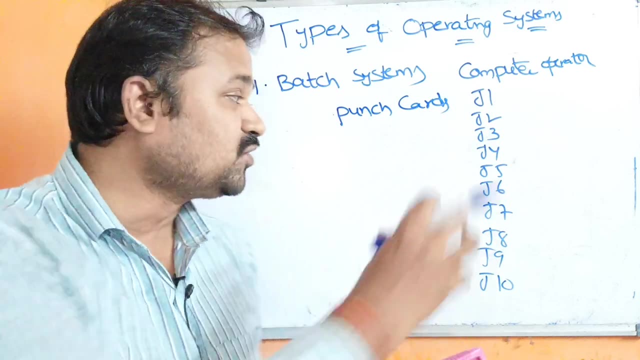 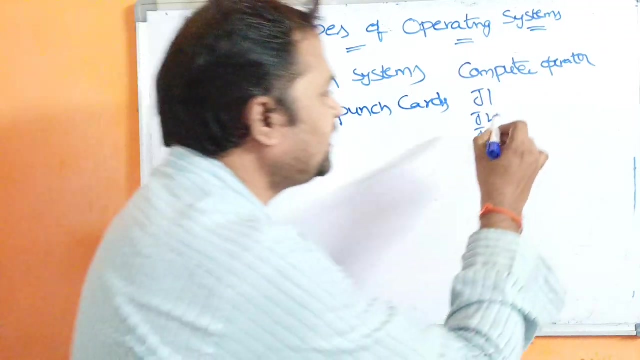 punch card. okay, in punch card that information will be available. okay, and after that what the computer operator will do is: computer operator will group all these jobs into batches according to the requirement. okay, okay, let us assume that the first five jobs are executed using cobalt programming language, so the 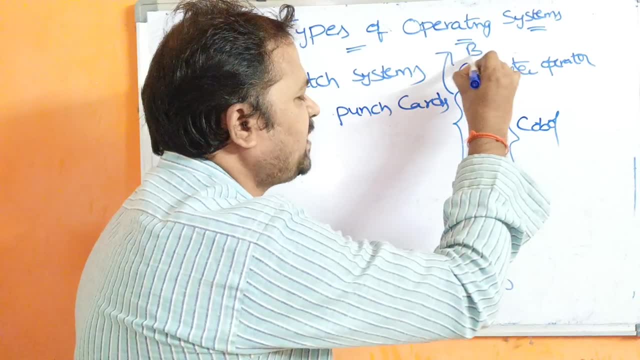 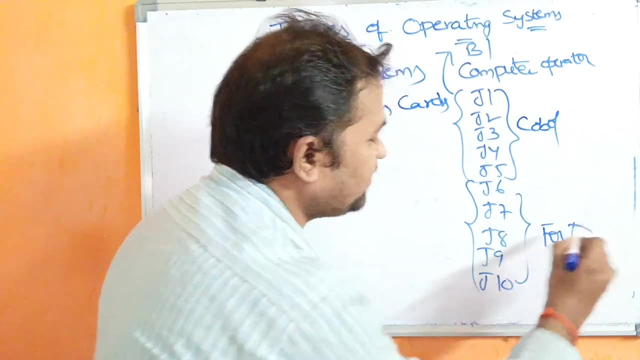 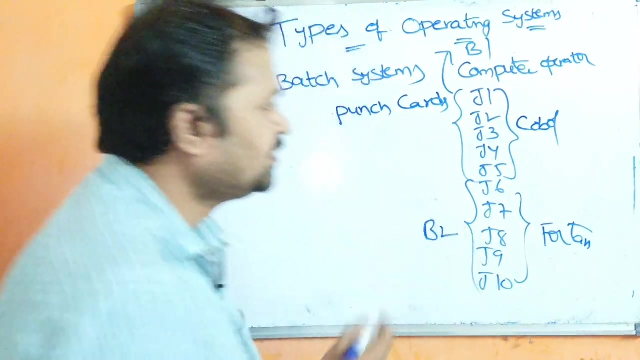 first five jobs will be grouped into a batch called b1. let us assume that the next five jobs are implemented using fortran language- fortran language. so the computer operator will group all these jobs into a batch called b1. so first computer operator will provide b1 jobs information. 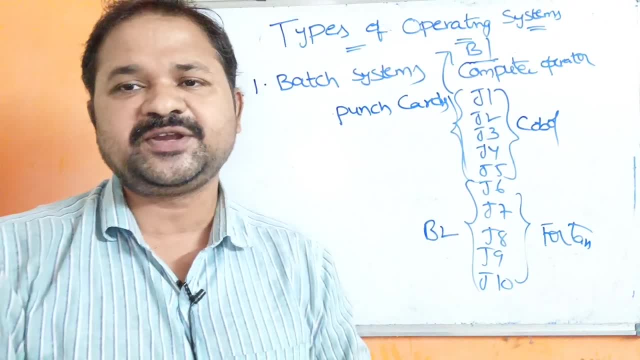 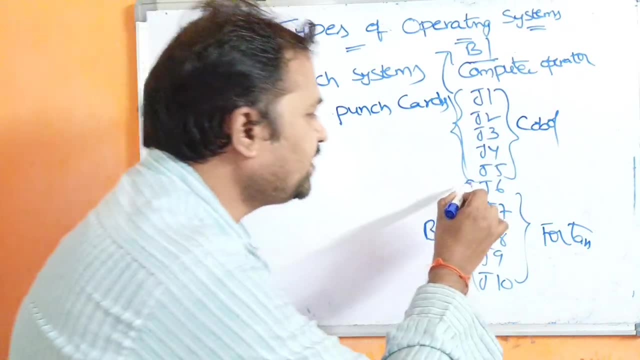 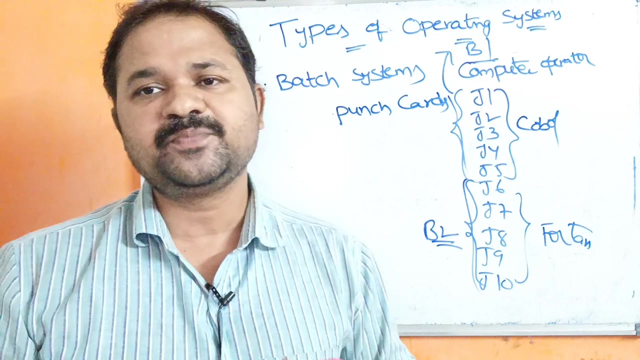 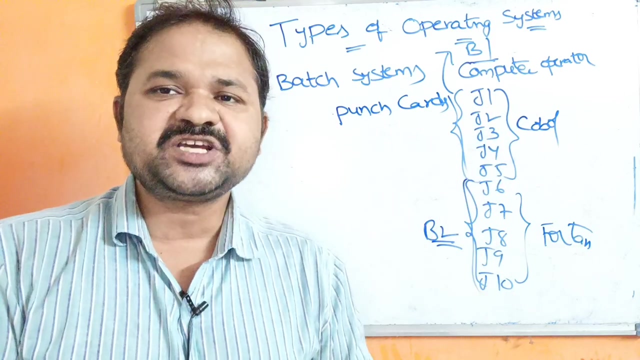 to the computer. now it is the responsibility of the computer to execute b1 jobs. okay, and after producing the output, the computer operator will supplies batch 2 information to the corresponding computer. okay, so computer will executes and produces the given and produces the output to the user. but the major problem with this approach is that let us assume that cpu is executing- 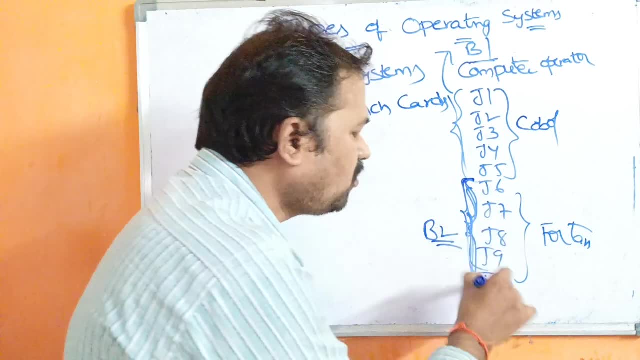 b1 jobs and after producing the output the computer operator will supplies batch 2 information to the user. but the major problem with this approach is that it is not working according to the requirement but b2 jobs and assumes that all these jobs are waiting for some ivo operations during ivo operation. 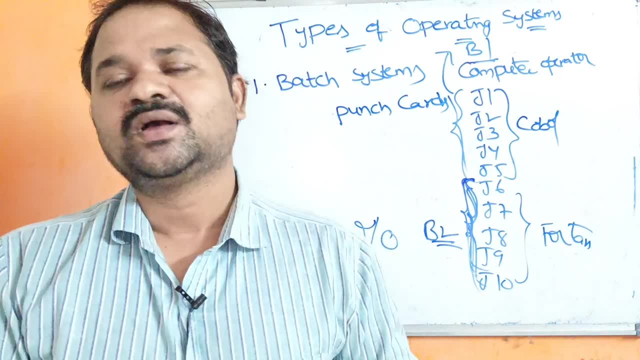 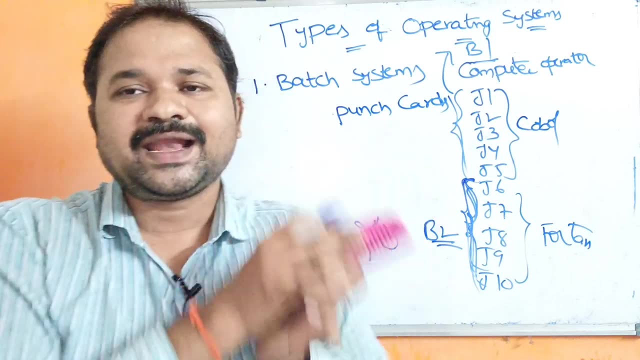 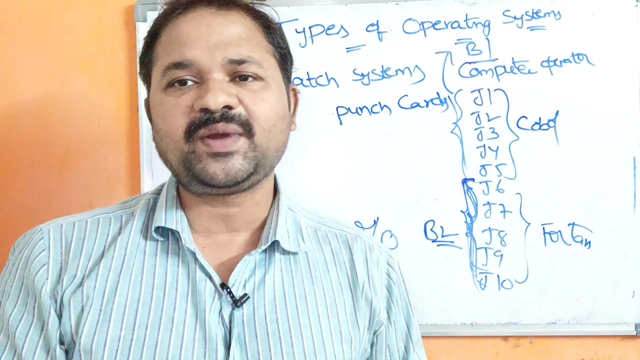 cpu will city as ide, but during that time it is not possible to allocate operating system to some other batch. so when operating system allocates cpu to some other batch only after completing execution of these batches, then only operating system allocates cpu to some other batch. okay, so 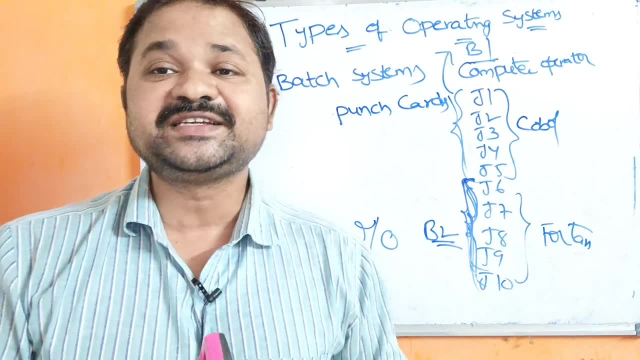 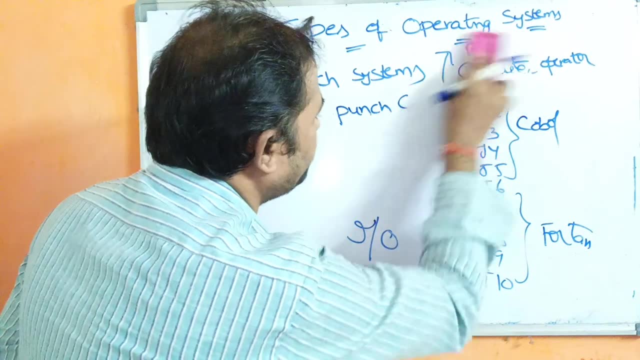 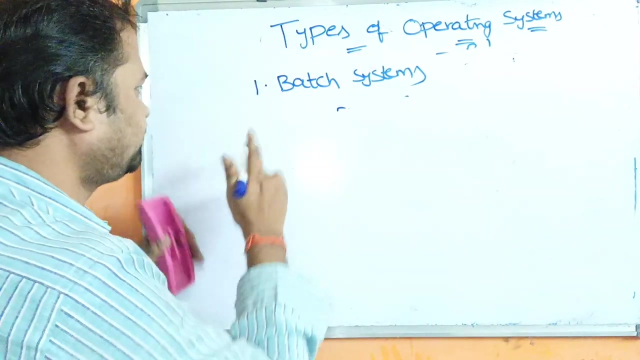 this is the problem here: most of the time cpu will see as id okay while doing the io operations. we can overcome this problem with the help of second type of system, that is, multi-programmer system. so the second type of system is multi-programmer system. multi-programmer system. 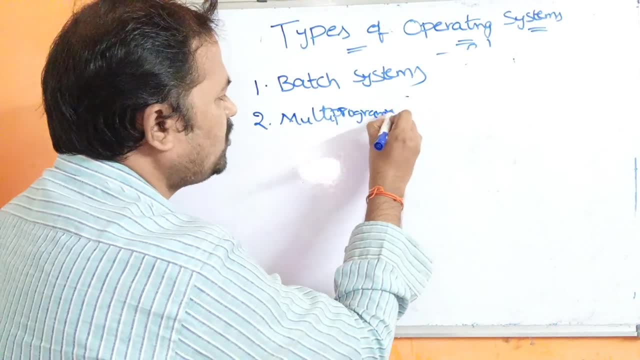 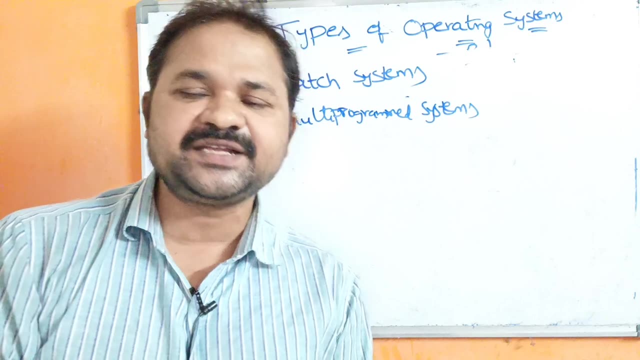 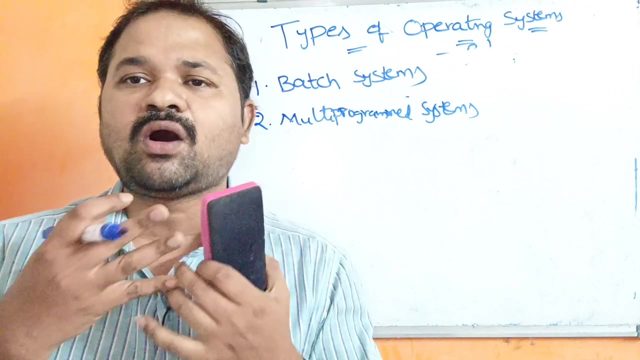 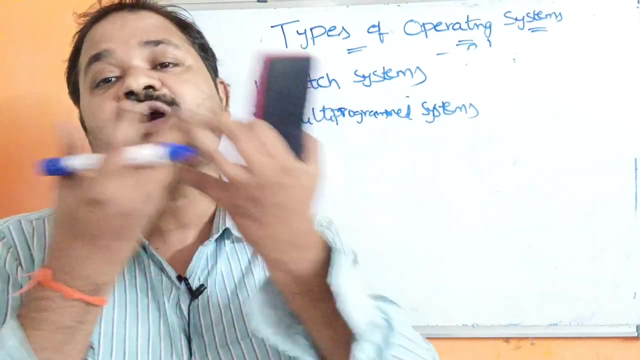 the name itself specifies the meaning. so what is multi-programming? multi-programming means placing multiple programs. multi-programmer system means we can place multiple programs in the main memory and we can execute all the programs simultaneously. so that is about what is multi-programming: keeping more number of programs in the main memory and executing all those programs simultaneously. the major advantage of this approach is cpu utilization. cpu utilization: we can utilize the cpu in effective manner if we use multi-programming operating system. let us assume that in main memory we have three processors are there, so p1, p2, p3- three programs are there. 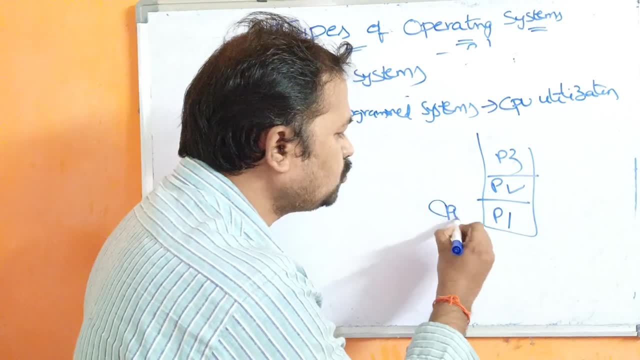 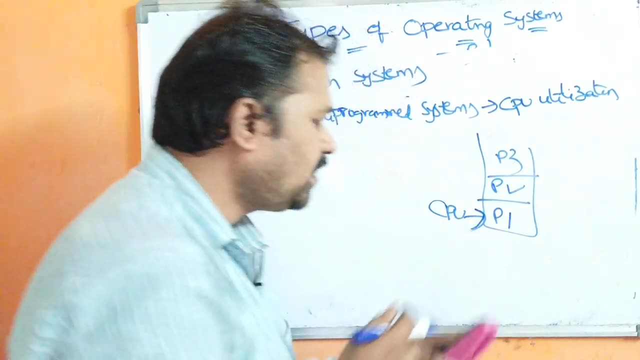 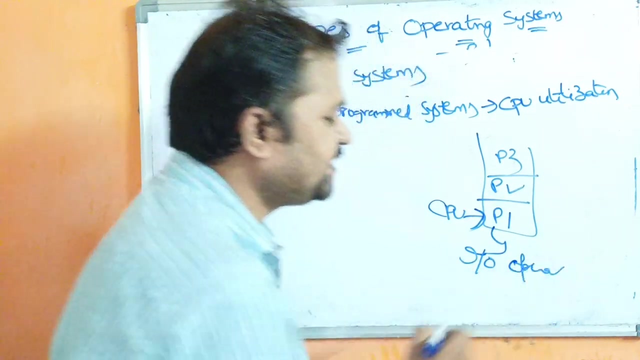 let us assume that operating system allocates cpu to process p1. so now cpu is executing p1 and and after some time assumes that p1 needs some iowa operation program. one needs some iowa operation. so during iowa operation there is no need of cpu. cpu will sit as ideal. so what the cpu will do is: 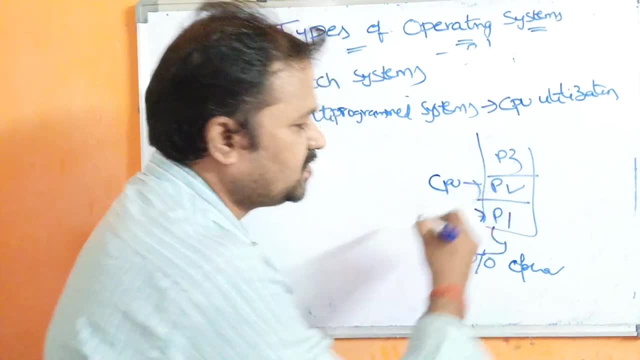 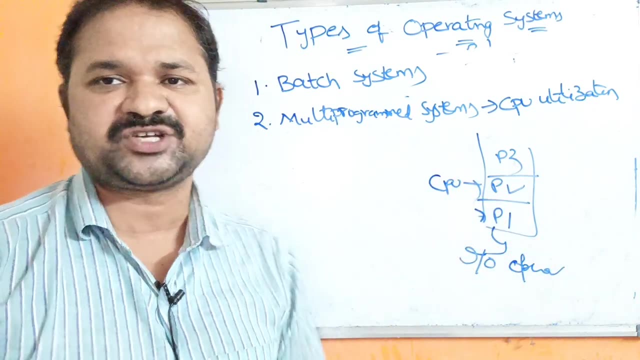 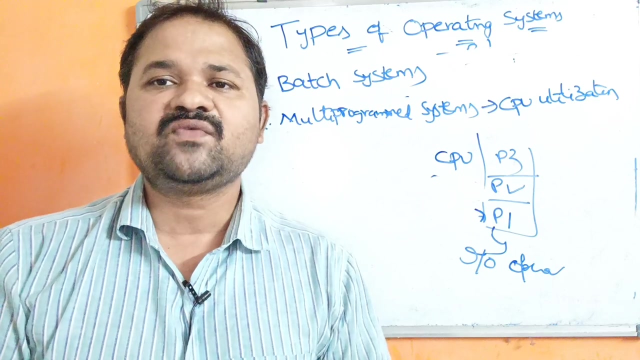 cpu control will be shifted to second program now. so now cpu starts executing process p2. okay, let us assume that p2 also requires some iowa operation. so operating system allocates cpu to some other process. so this is the advantage here: while one process is waiting for some iowa, 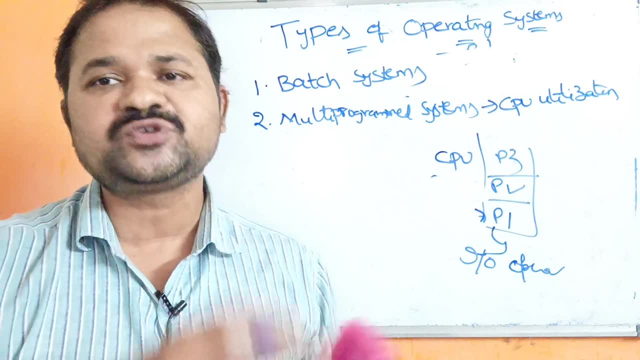 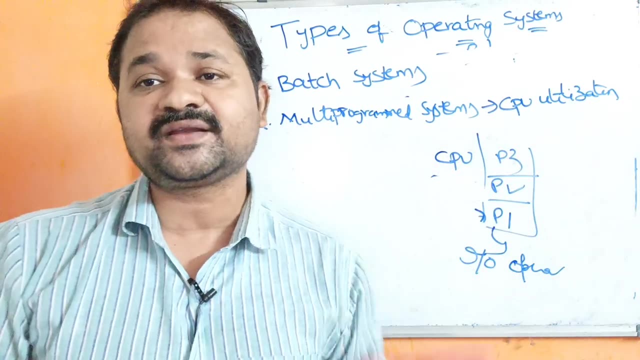 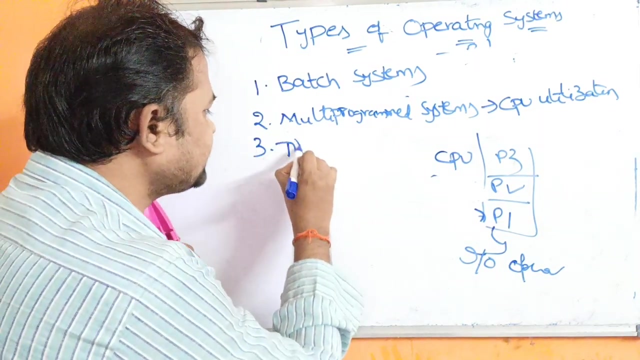 operation operating system allocates cpu to some other process. so likewise we can utilize the efficiency of the cpu in effective manner with the help of the multi-programming system. now let us see the third type of system, that is, time sharing system. so the third type of operating system is: 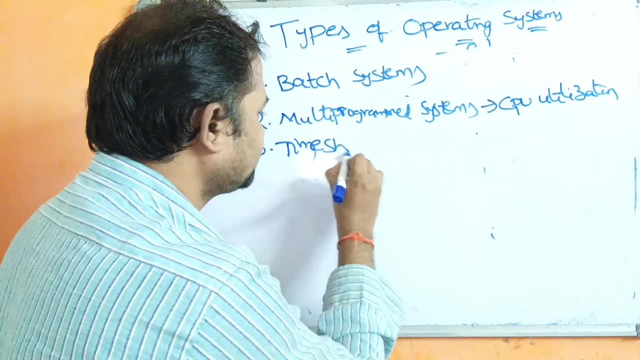 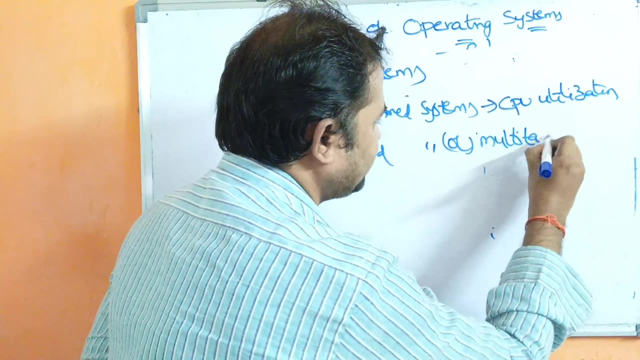 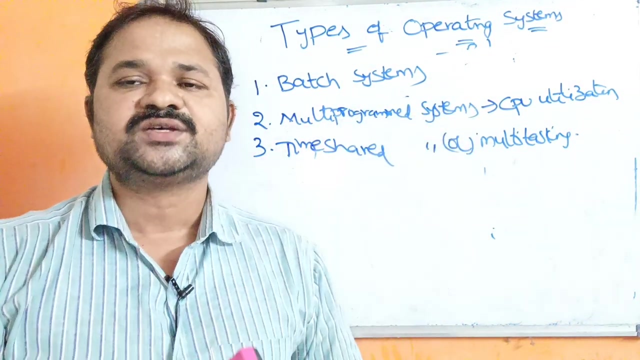 time sharing system or time sharing systems. so time sharing system or this can also be called as a multitasking system, multitasking so here. so time sharing means it is an extension to the multi-programming system. so here also, main memory may contain multiple programs and all those. 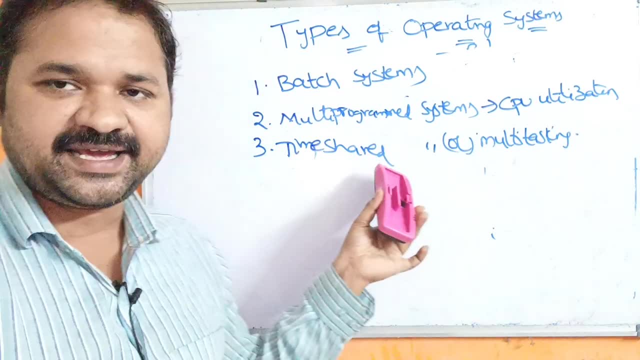 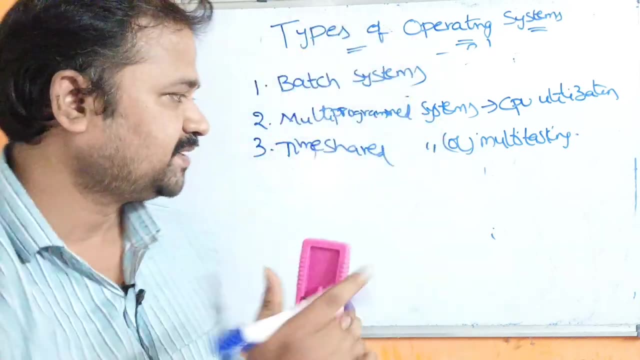 programs are to be executed simultaneously. time sharing- the name itself specifies the meaning. cpu allocates a time to all the processes. let us assume that three processes are there in the main memory. so time sharing means it is an extension to the multi-programming system. so here also main. 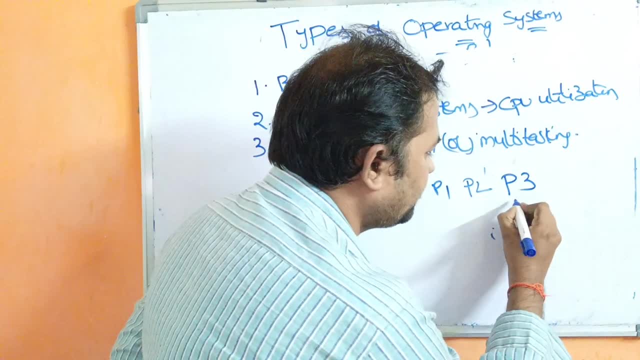 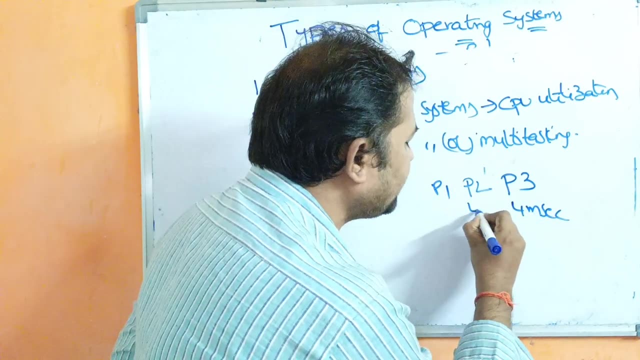 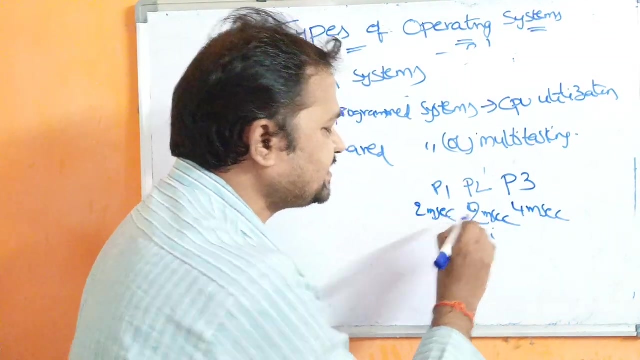 memory may contain multiple processes. so p3, p2, p1. three processes are there in the main memory let. for executing p3, it requires four milliseconds. for executing p2, it requires two milliseconds of cpu. for executing p1, it requires- let us assume that- two milliseconds of the cpu. okay, here assumes: 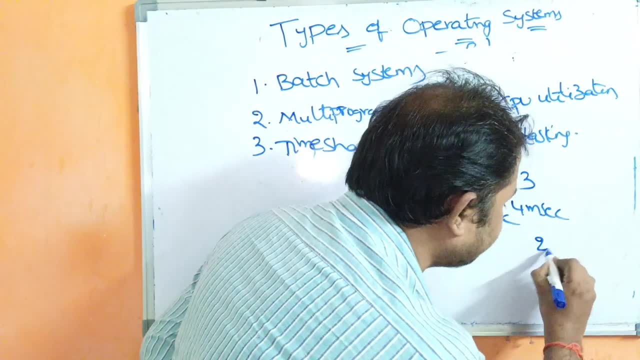 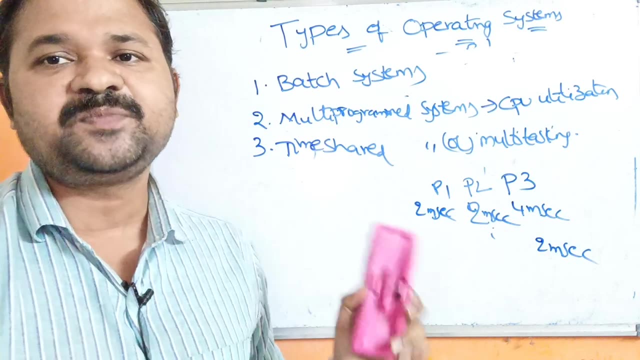 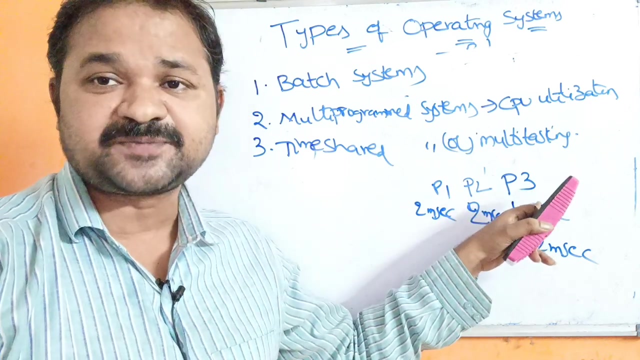 that operating system allocated two milliseconds to all the processes. operating system allocated two milliseconds to all these processes. so cpu can allocate each process only for two milliseconds only. so assumes that first cpu starts executing process p3. so here what is the time? here four milliseconds, but cpu can execute only up to 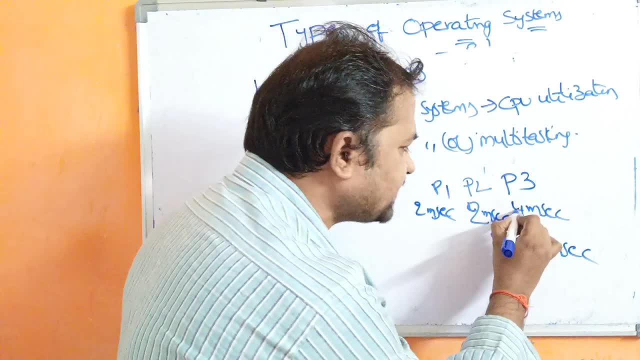 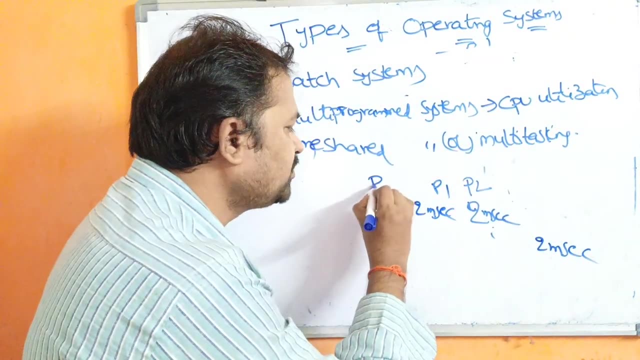 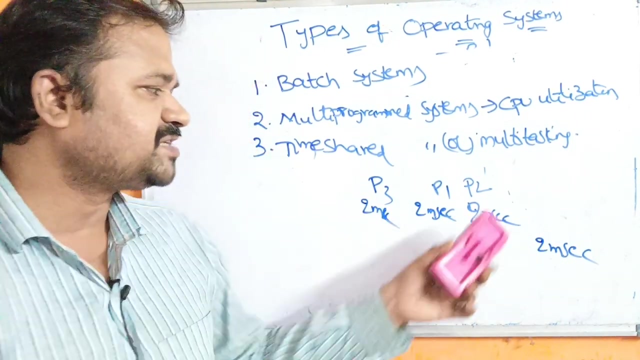 two milliseconds only. so p3 executes to two milliseconds. so remaining time is two milliseconds. so the remaining? so that process will be appended to the end of the list. okay, beginning of the list. okay, so what is the remaining time? two milliseconds. so now cpu executes p2. so p2 requires only two milliseconds. so there is no problem. so cpu. 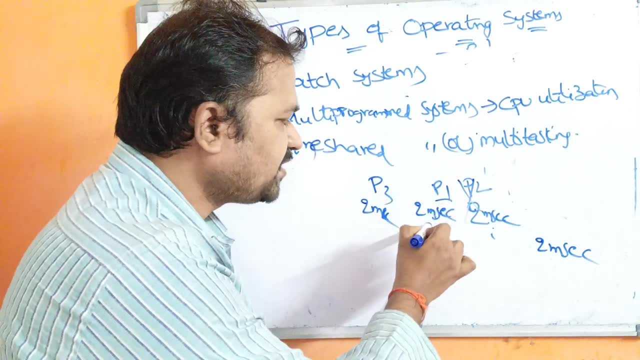 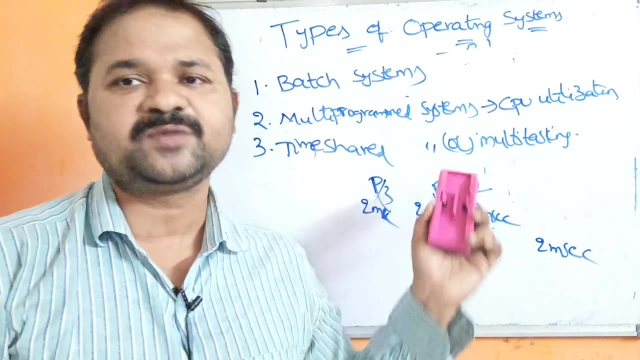 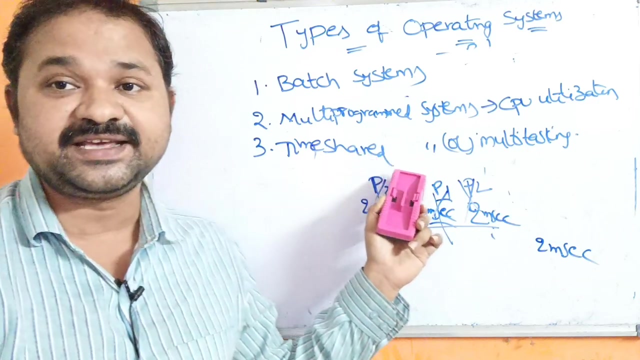 completes the execution of the p2 next to p1 also requires two milliseconds. so cpu also completes two milliseconds next to cpu completes p3: two milliseconds of the p3. so now we can conclude that all the processes completed their execution. so this is about time. sharing system, so a time. 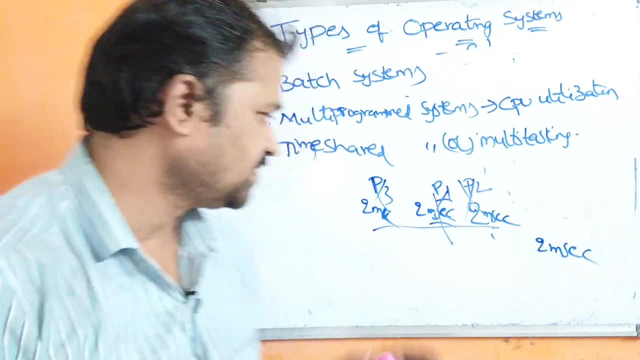 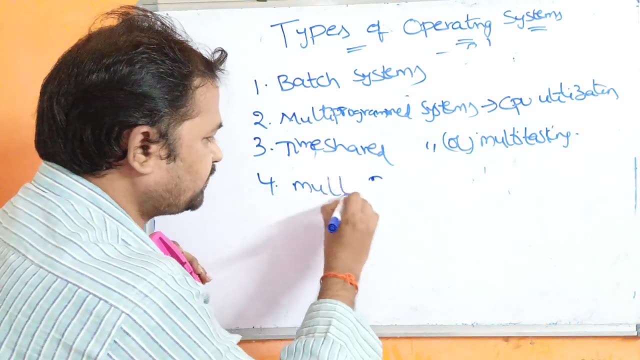 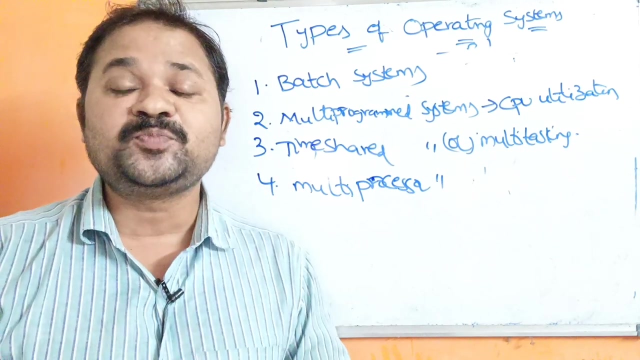 will be shared among all the processes that are in the system. now let us see the next one, that is, multi processor system. multi processor system, so multi processor system. the name itself specifies the meaning. instead of single processor, multiple processes are collected to the same computer. so here we have a single computer. let us assume that. 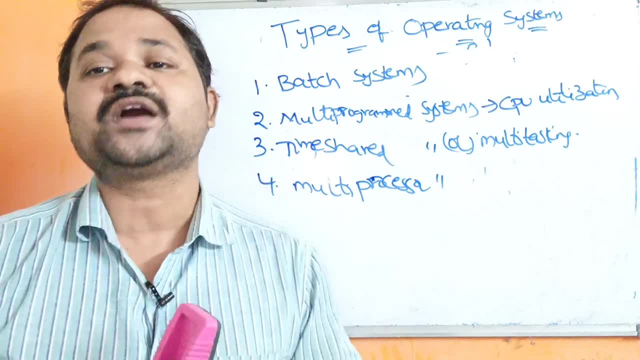 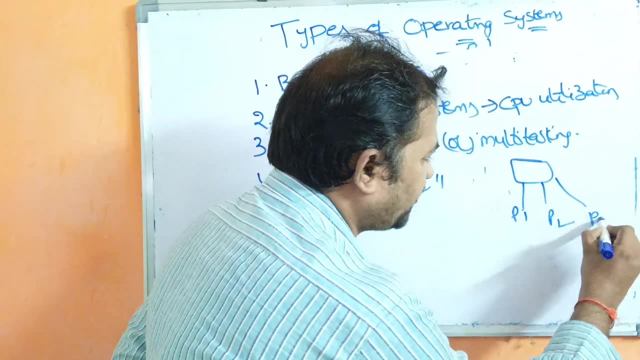 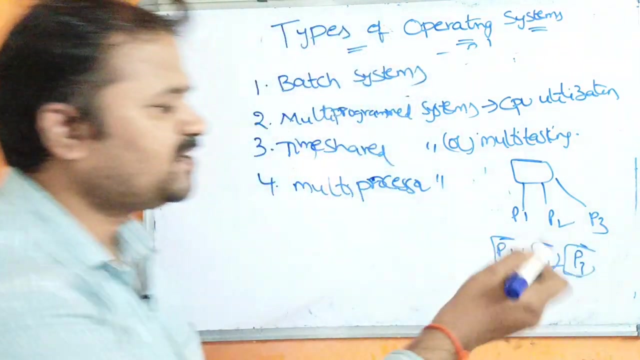 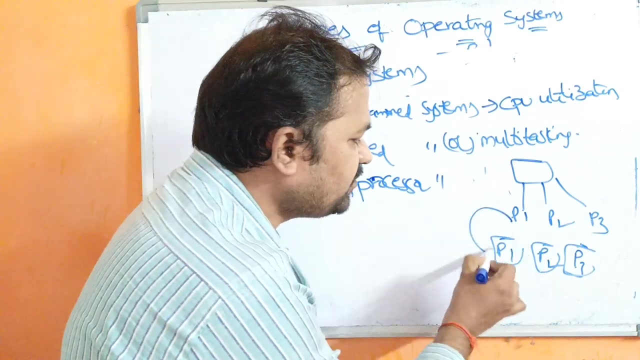 three processors are connected to the corresponding computer. so we have a single computer with three processors. this is p1 processor, p2, p3 processor and assumes that we need to execute three processes. we need to execute three programs, so p1, p2, p3. so we need to execute these three processes. now what will happen? p1 will execute. 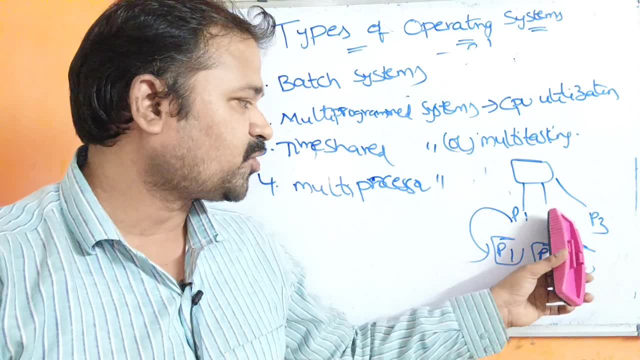 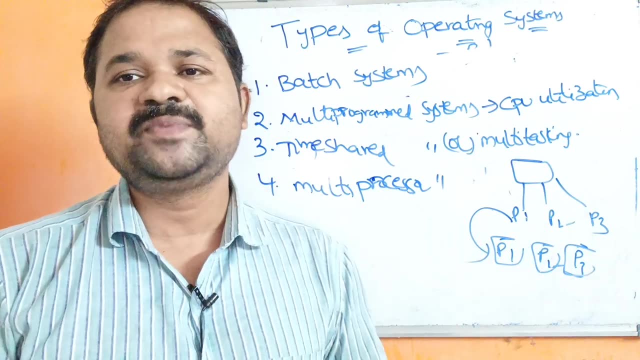 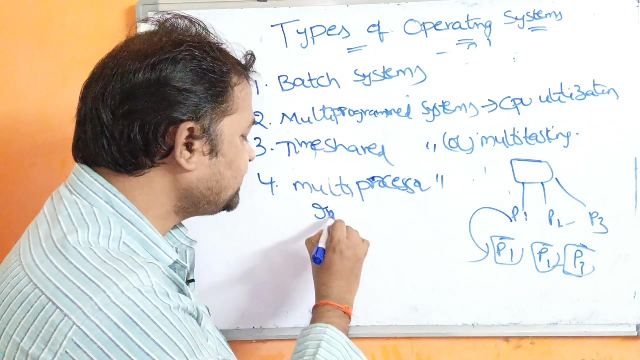 processor 1 will execute p1 program. processor p2 executes p2. processor p3 executes p3 program. so all these three programs will be executed concurrently. so what will happen? it increases the output. so there are three advantages, are there? the first advantage of multi-processor is 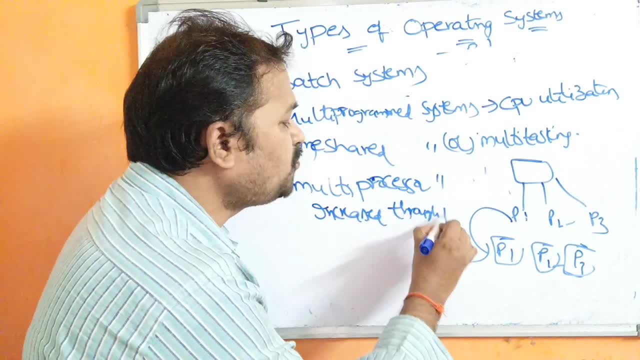 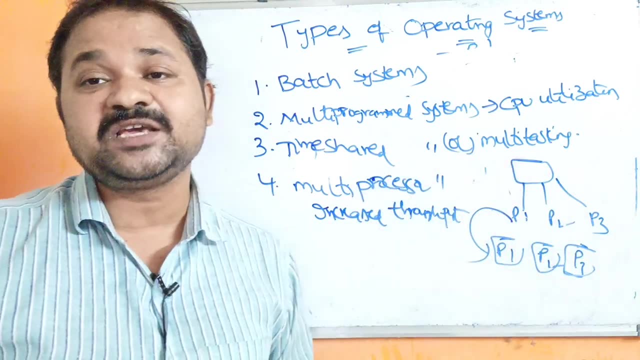 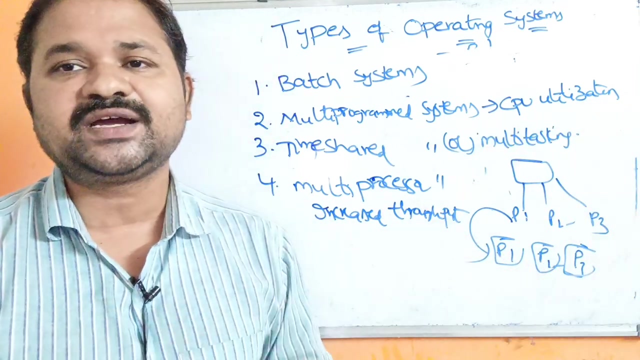 it increases the throughput. so throughput means output will be increases. in less span of time we will get the output, whereas if we have only one cpu, then that cpu has to execute all these three processes concurrently. instead of that, here we have three processors are there, so that in less 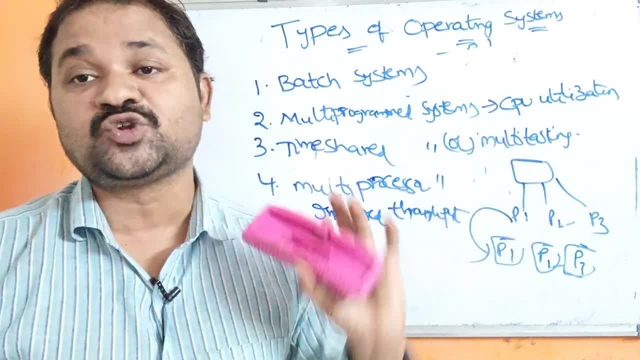 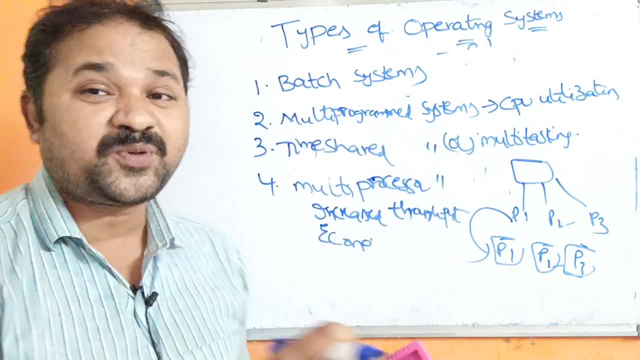 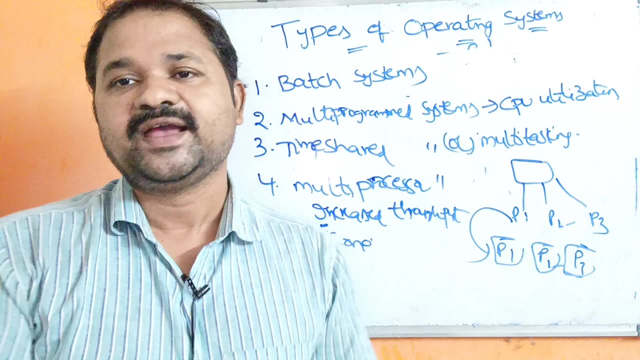 span of time we can get the output. so increases the throughput. and the second advantage is economy. it is very, very cheaper process. why? because three processors are attached to the single computer only here we are not using three different, three separate computers. instead of that we are using only a single computer and three processors are attached to that computer. so it 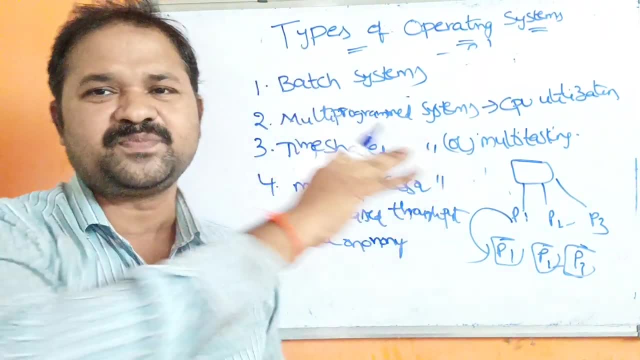 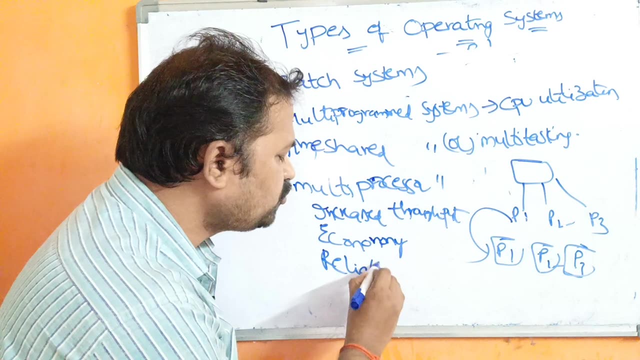 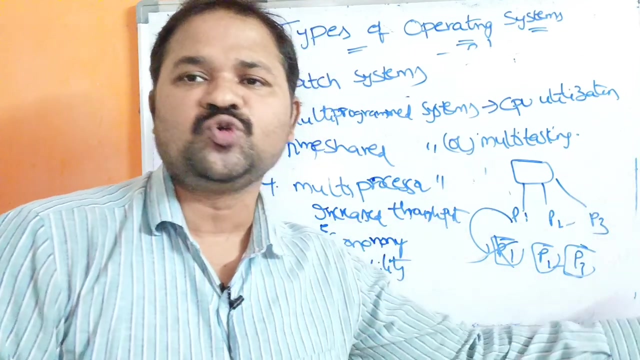 is very, very cheaper, okay, when compared with the three computers with three processors. okay. and one more advantage is reliability. suppose due to some problem, if one of the processor fails, then there is no problem, the remaining processor will come, the remaining two, one of the one of these. 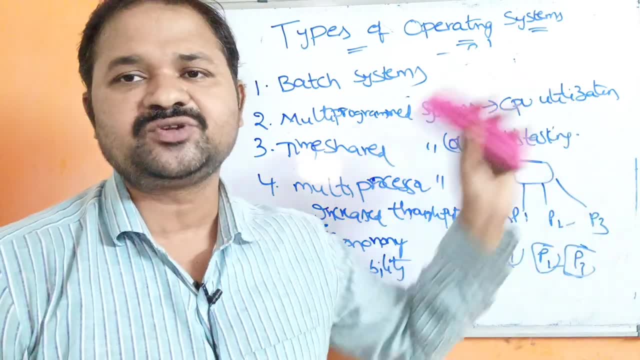 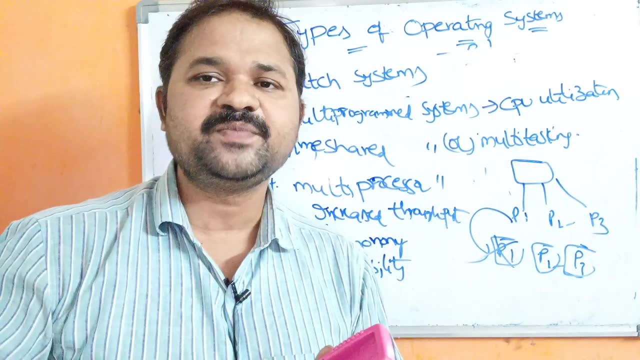 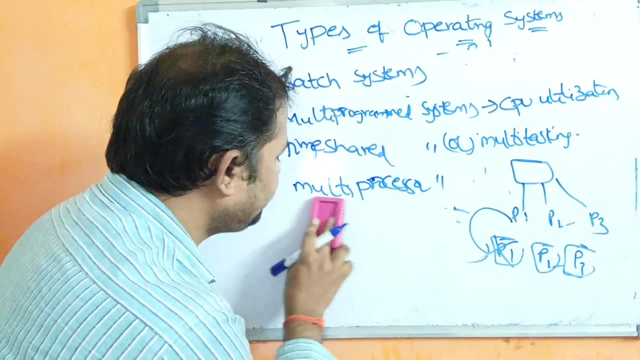 two processors will come into the picture and execute the corresponding uh process. okay, reliability, okay. if one processor fail, then there is no problem, the remaining processors will execute the corresponding task. so this is about multi-processor system. multi-processor system. now let us see the next one, that is, distributed system. distributed system. 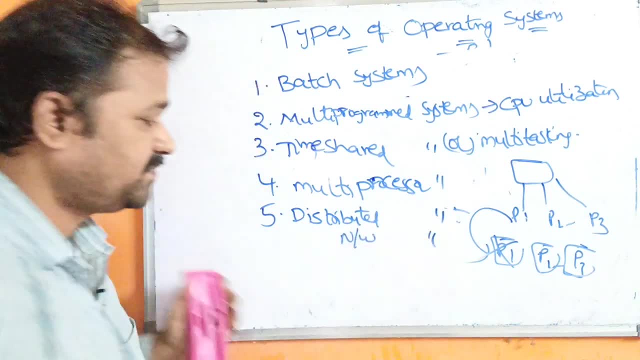 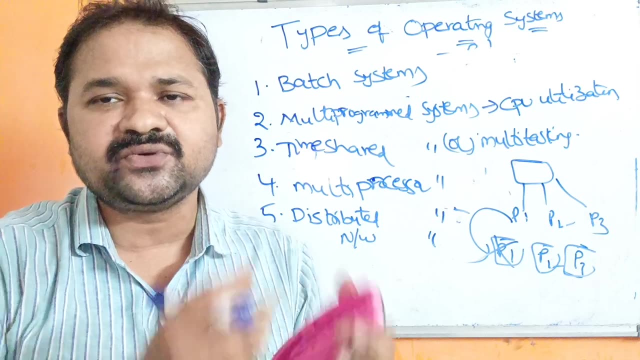 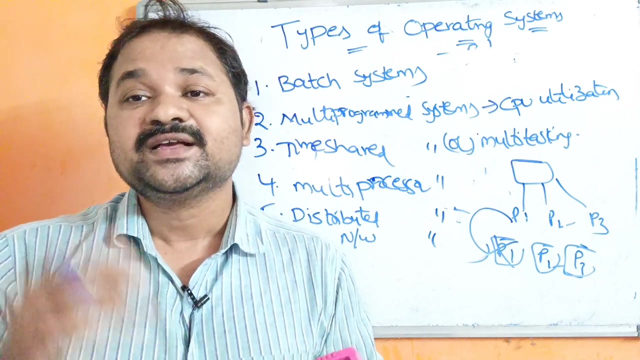 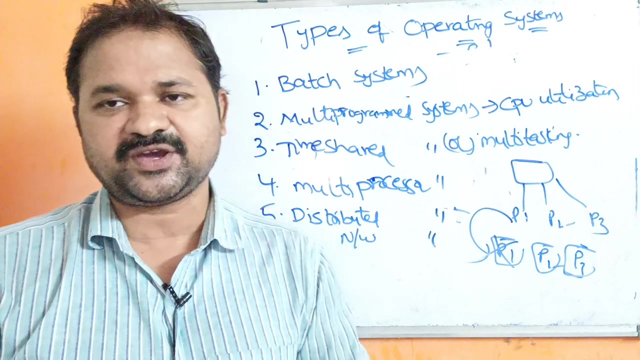 distributed system can also be called as network system, distributed system. the name itself specifies the meaning. the same information will be distributed to all the systems in the corresponding network. let us assume that 10 persons are working on a same project. let we have a network with 10 systems. assumes that 10 persons are working on that project. okay. 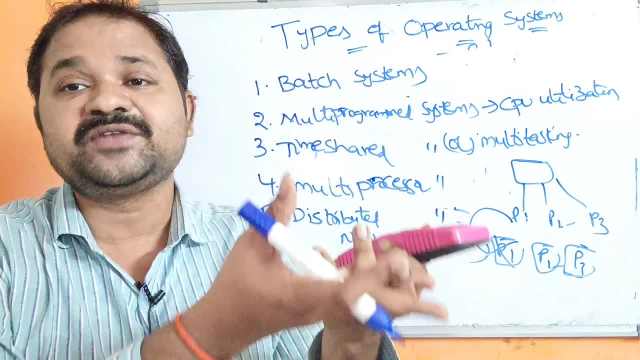 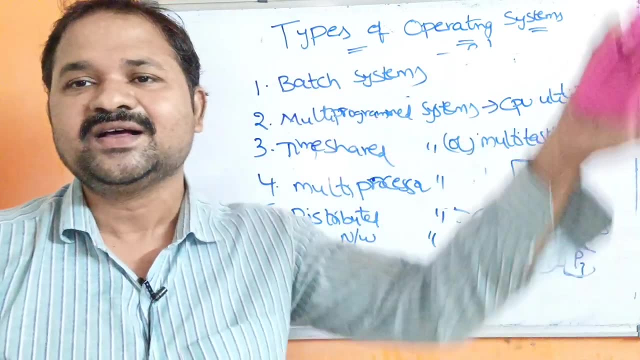 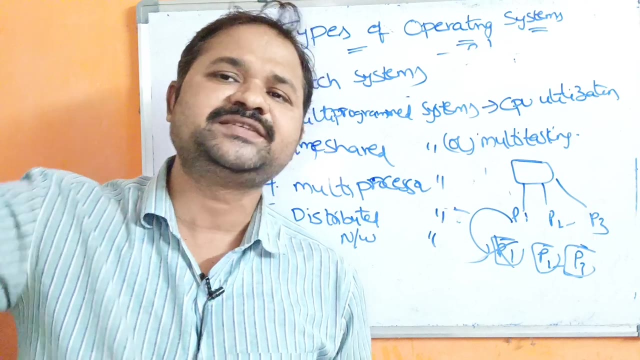 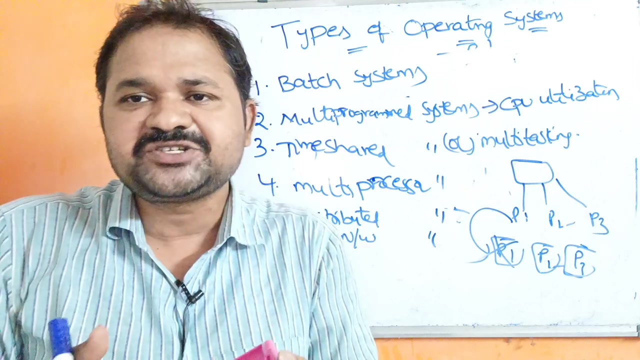 so then, what will happen is that information, that problem information, that project information will be distributed to all the 10 persons. let us assume that p1 has designed the first two modules, so those two modules code will be distributed to remaining all nine nine systems. also assumes that p2 designed module 3 and module 4, so that information is. 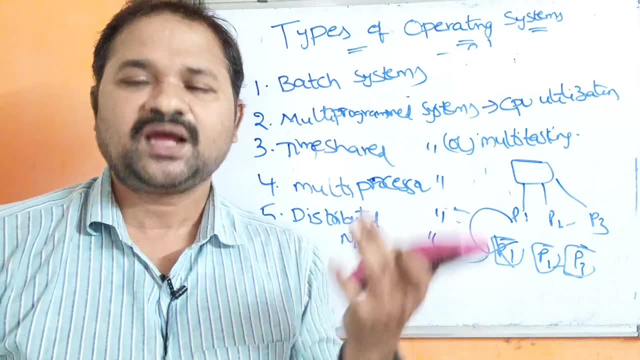 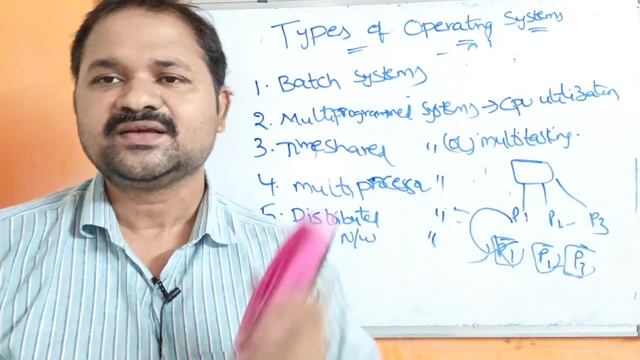 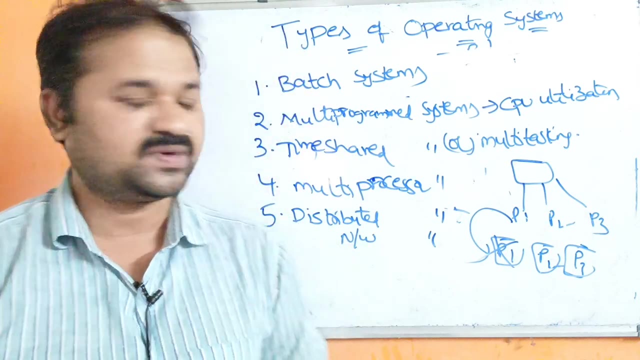 distributed to all the systems also due to some problem, assumes that the first computer and the it is failed, then there is no problem. why? because those copies are already available in the remaining nine computers, so there is no problem. so this is about distributed system or network system. 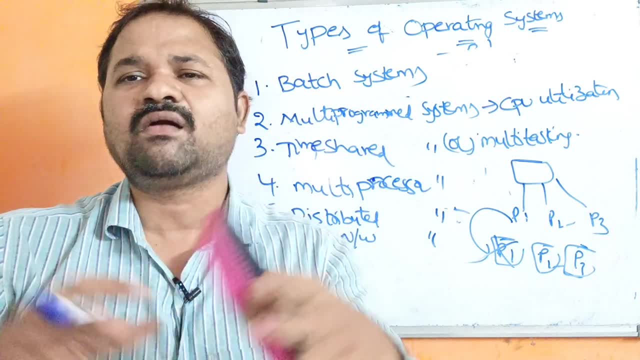 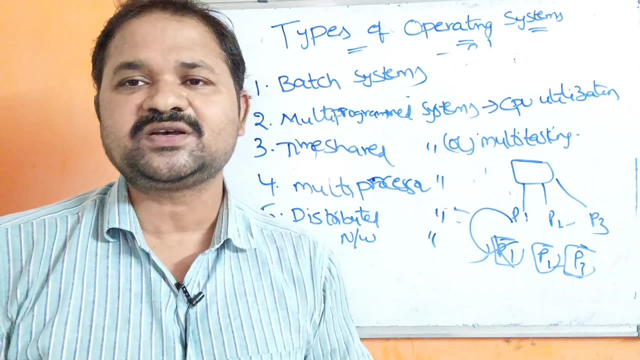 so that same information will be distributed to remaining all the systems in the network. so, due to any problem, if one or multiple systems fail, then there is no problem. why? because that same data is replicated in all the systems also, that's that same data is available in all the. 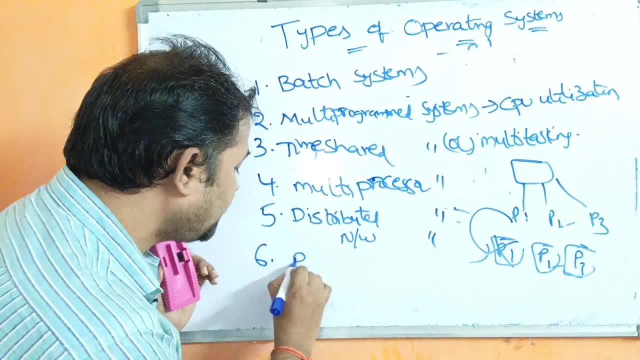 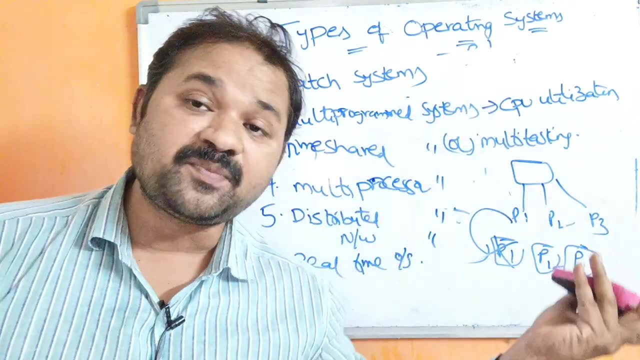 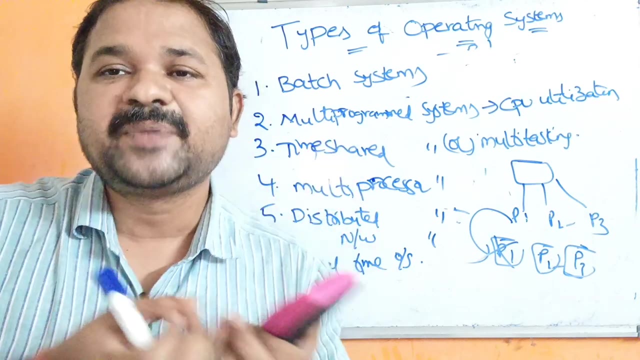 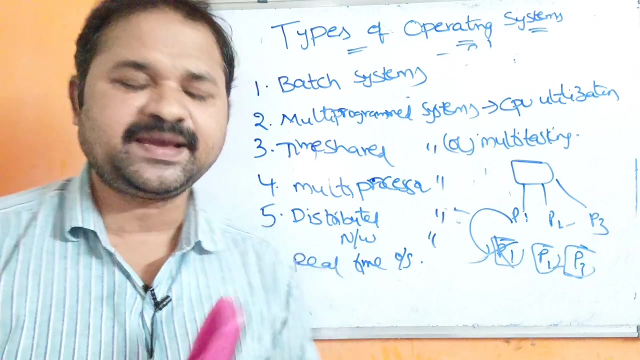 the systems also, and we have one more system called real-time system. real-time operating system is mainly useful in order to implement real-time applications. real-time applications: if we want to perform an application in a specific period of time, in a specific amount of time, then we have to use real-time operating system. there are two types of real-time operating systems are: 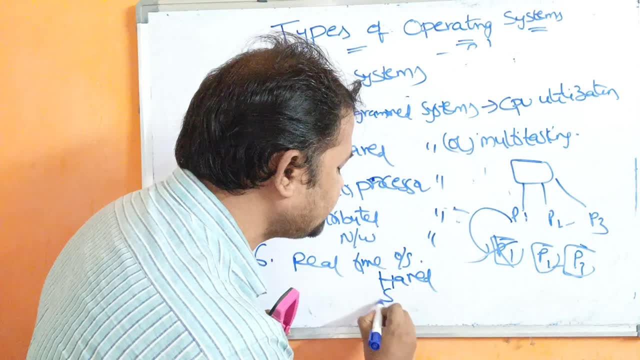 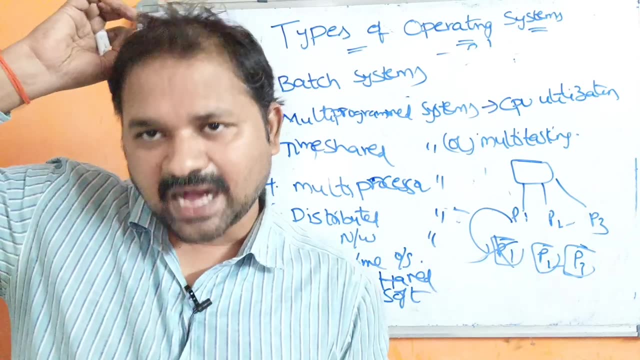 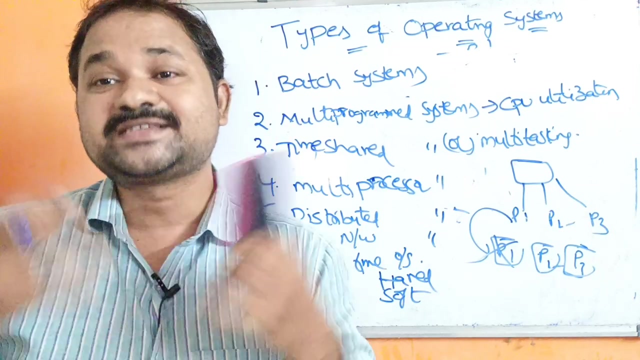 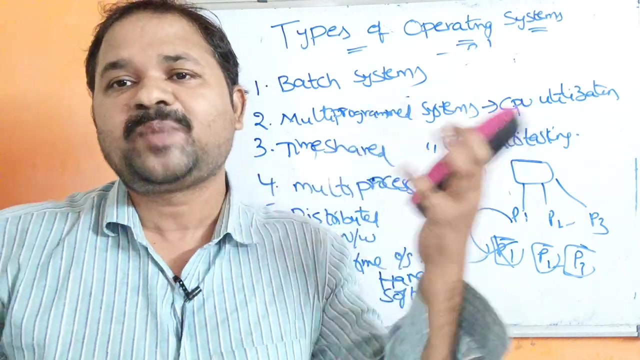 there. first one is hard real-time operating system. second one is soft real-time operating system. hard real-time operating system means that application should be executed within that stipulated amount of time only. otherwise the system will fail. the best example for the hard real-time application is if we take a aeroplane driving. okay, the pilot will drive based upon the